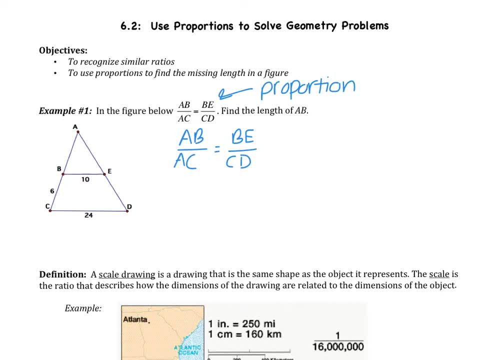 The CD is a ratio. Now all you have to do is plug in what you know. Well, AB, I actually don't know that. Let's call it X over AC. Well, AC, is this whole portion right here? It is not 6.. 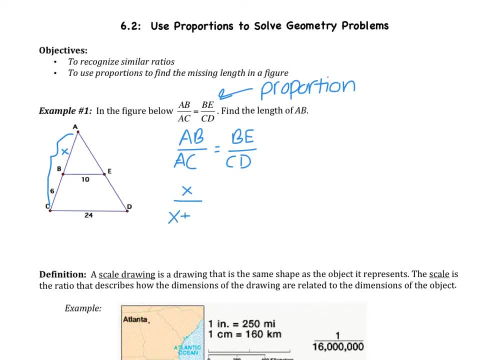 Let's be aware that it's X plus 6.. That's a very common mistake, so please watch out for that. It would equal Well, BE is 10, and CD is 24.. Now you have this proportion. next step would be to cross multiply. 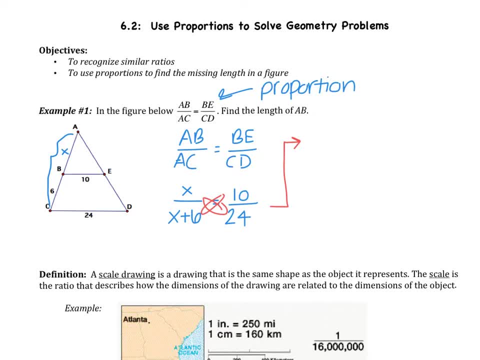 Now when you cross multiply, you have to make sure you distribute properly. So you would get 10 times X plus 6, would equal 24 times X. Make sure you distribute your 10. It's really 10X plus 6.. 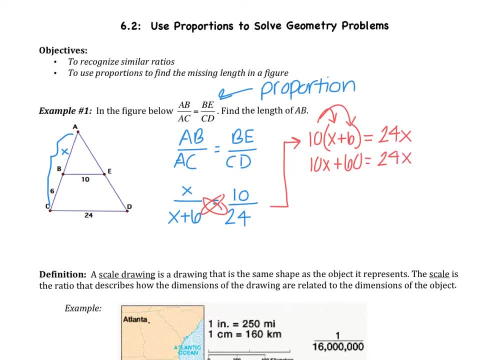 plus 60 equals 24x. you would get then that 60 equals 14x. divide by 14,, divide by 14, x would be 30 over 7.. That's great, we know x. Now let's answer the problem. 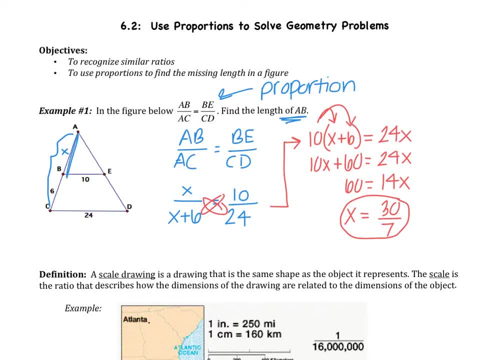 The problem says: find the length of AB. Well, in this case AB is x. so even better, Remember AB would equal 30 over 7.. Okay so proportions are actually pretty easy. Just make sure you plug in the correct values as you go. 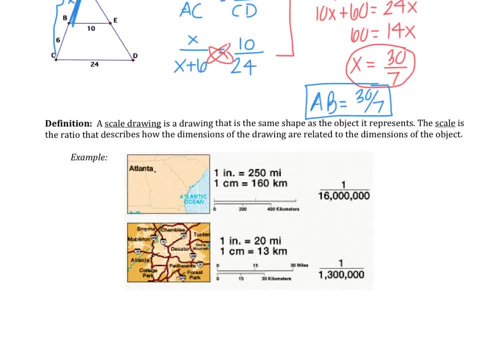 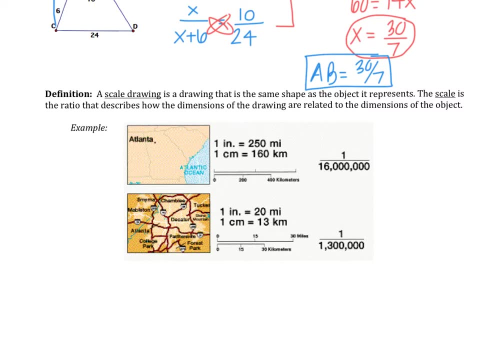 Moving on. then we have a definition of what a scale drawing is. So a scale drawing is a drawing that is the same shape as the object it represents. The scale is the ratio that describes how the dimensions of the drawing, or related to the dimensions of the object. 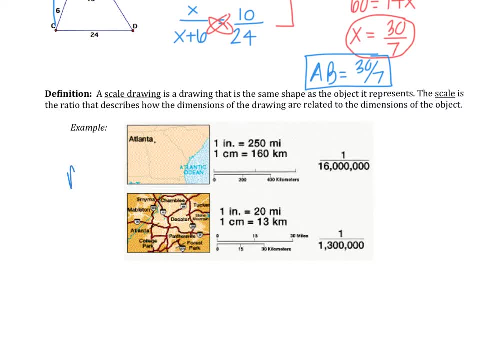 Now a really good example of a scale is in a map which is shown right here. It says one inch on a map is really 250 miles in real life. For the next one, it says one inch is really 20 miles in real life. 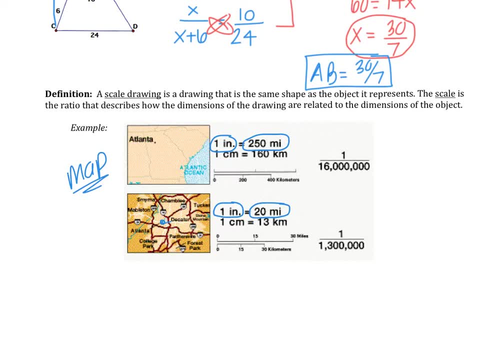 So, for example, if I measured, maybe like this city to this city, and I found that this city is really 250 miles in real life and I found that this city is really 250 miles in real life and I found that this city is really 250 miles in real life. 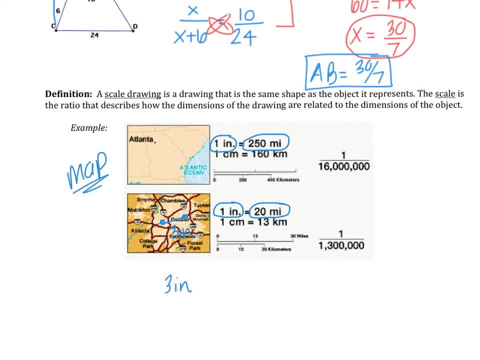 and I found that it's three inches. well, three inches in the picture really is 60 miles in real life. Again, you wouldn't be able to see 60 miles on a piece of paper. That's why you have a scale. 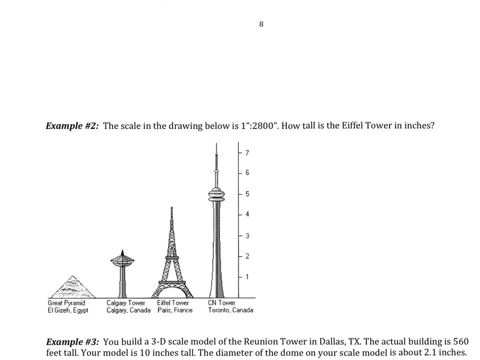 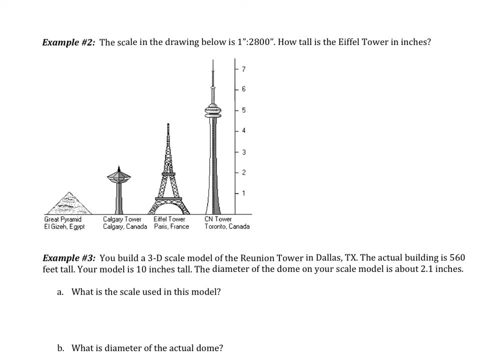 Using that. let's go to this next example. For example two: the scale in the drawing below is one inch to 2,800 inches. For example two: the scale in the drawing below is one inch to 2,800 inches. 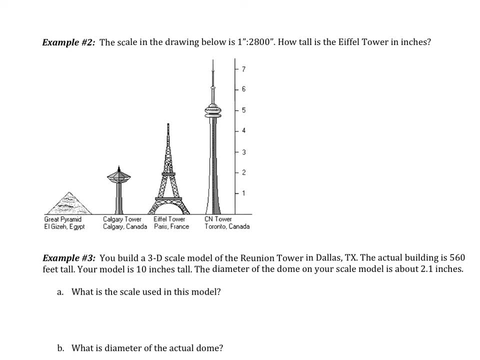 How tall is Eiffel Tower in inches? Well, to start off, this is the scale: One inch to 2,800 inches. You can think of it that way. Okay, it's the scale. Now we can set up the proportion to solve this. 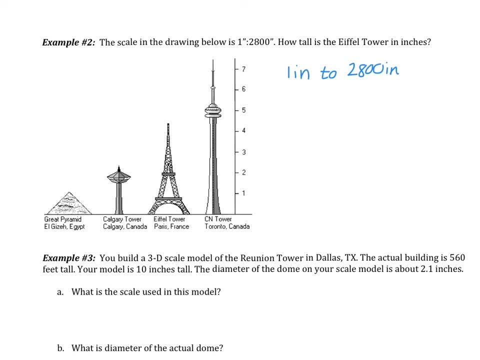 Okay, now, when we set up the proportion, it's important to be organized. I'm going to put the drawing on top. I'm going to put the drawing on top. I'm going to put the drawing on top. Then, on the bottom, is the real life size of it. 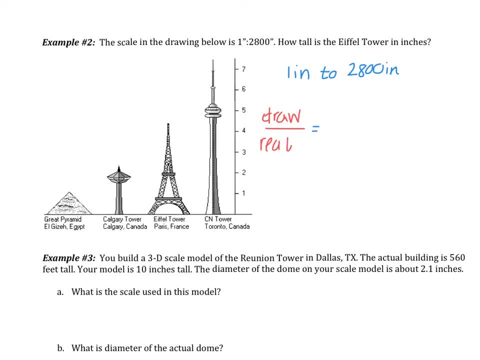 Then on the bottom is the real life size of it. So in- Sorry, I'm going to erase that, Sorry, I'm going to erase that. So that's just labeling what I'm going to be using. So I have one inch over real life is 2,800.. 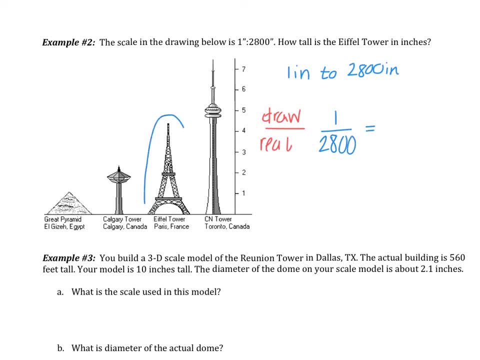 Now I have to use that to find the drawing. Well, the drawing here. if I go across, I might say about 4.5 inches, 4.5 in the drawing. Let's find out what that would be in real life. 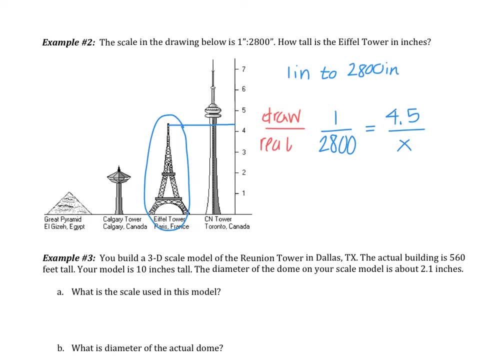 Put that over x, So the drawing is all on top and the real world measurements are on the bottom. You need to keep that consistent. Then, when you cross multiply, you get x to be 12,600 inches. So that is how tall the Eiffel Tower is. 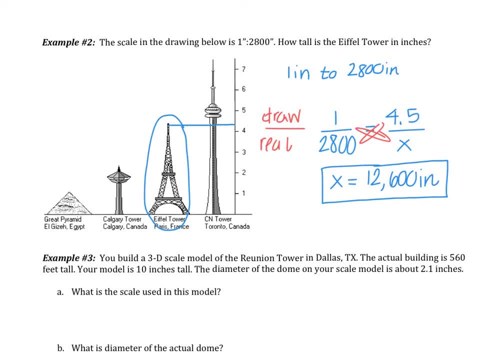 in inches. in real life, Obviously, the picture would not be able to be shown for 12,600 inches, so that's why we use this scale. Now, number three: You build a 3D scale model of the Reunion Tower in Dallas, Texas. 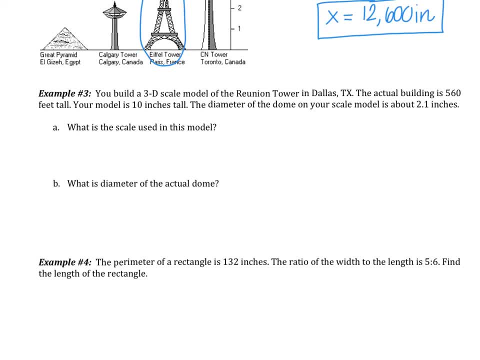 The actual building is 560 feet tall. Your model is 10 inches tall. The diameter of the dome on your scale model is about 2.1.. Please take a moment pause. try this one out on your own, So hopefully you had enough time. 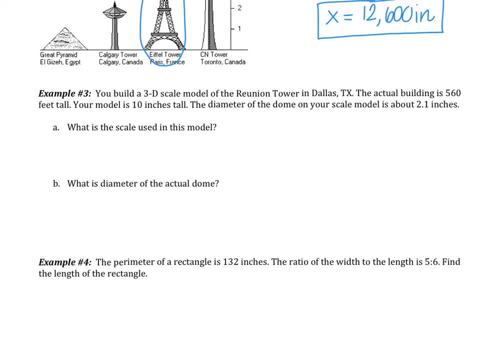 to give this one a try. First question is: what's the scale used in the model? Well, you have 560 feet tall to 10 inches tall. Well, there's your scale: 10 inches compared to 560 feet. Now, you always want to simplify your scale. 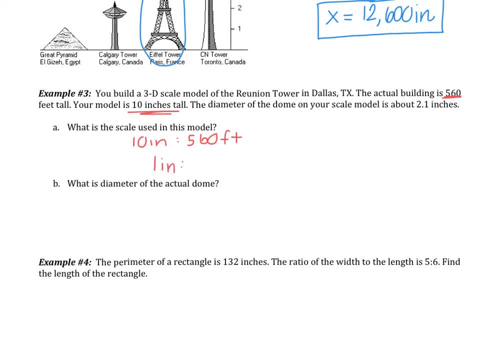 so please simplify it and the final answer should be 1 inch to 56 feet. That is your scale. Takes one inch in real- sorry, one inch on the diagram is 56 feet in real life. So now it actually wants you to find the dome. 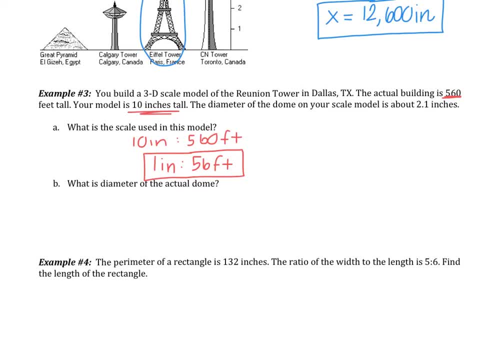 Again, you have to be careful about where your labels are. The first one: let's have the model, go on top and then we'll have the actual amount on the bottom. Okay, so we have our scale: 1 inch over 56 feet. 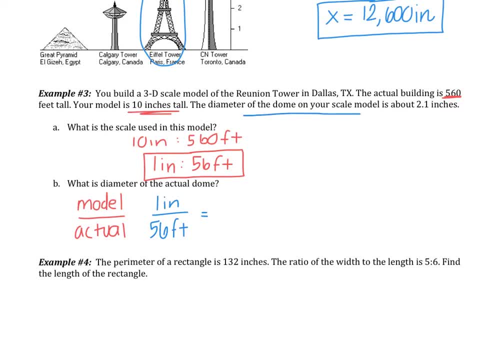 Now it says the diameter of the dome in your scale model is 2.1, which makes it 2.1 in the numerator, because the whole top is about the model. The unknown is on the bottom. Notice it's going to have a units of feet. 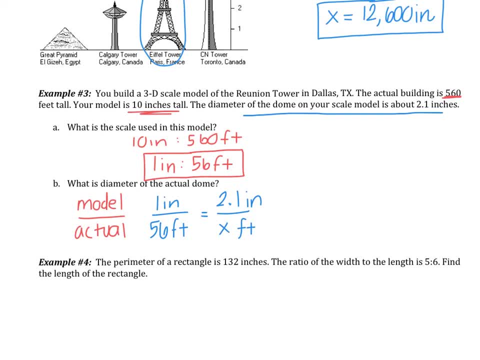 The actual is units of feet. The model is inches. Same idea: Cross multiply. When you do so, x would equal 117.6 feet. Keep in mind a scale can have different units. As you can tell, it went here from inches. 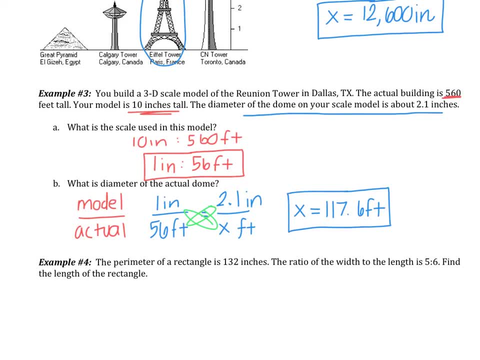 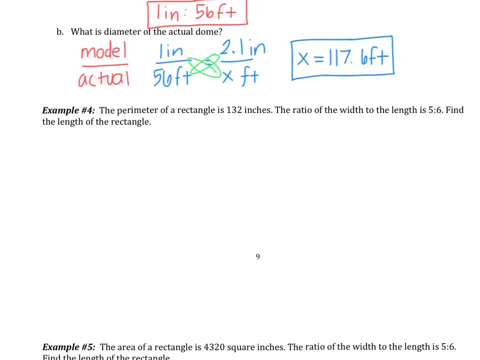 to feet. As long as you're consistent about it, you will be fine. Moving on to example four, The perimeter of a rectangle is 132 inches. The ratio of the width to the length is 5 to 6.. Find the length of the rectangle. 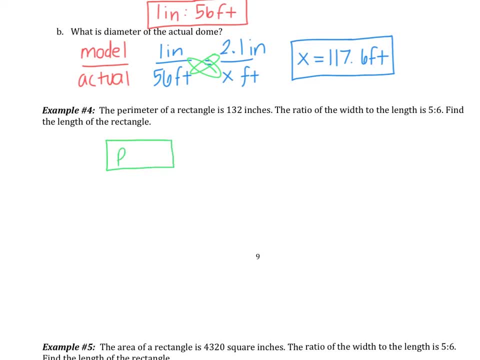 Once drawn out, here's my rectangle. The perimeter is 132 inches and it says I'm at a ratio of 5 to 6. It does not mean that the width and length are 5 and 6. It can't be. 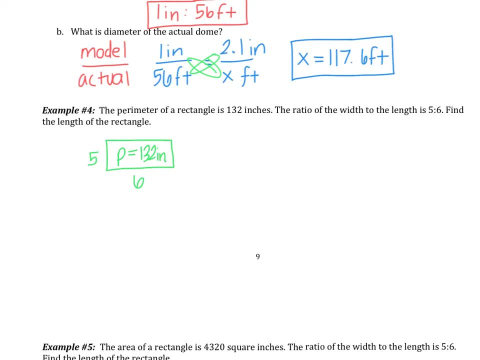 Otherwise your perimeter would not equal 132.. Get that idea out of your head. It means there's a common ratio. Really, there's a common value, x, that I took out to make this ratio Really the width and length. 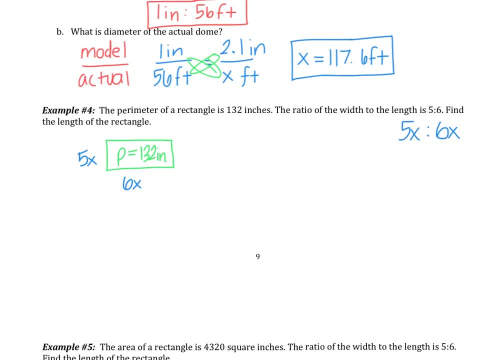 are 5x and 6x. Well, in a rectangle, opposite sides are congruent. So look at that. Now I can make an equation with my perimeter. Well, perimeter equals all my sides added up: 5x plus 6x plus 5x plus 6x. 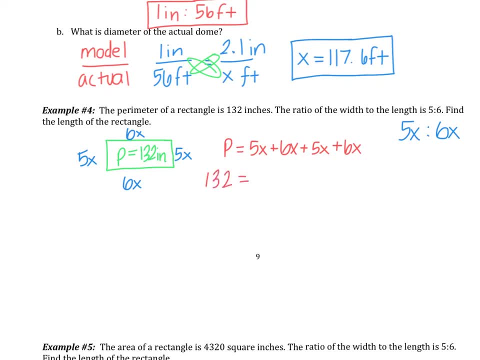 My perimeter, I know, is 132, and that equals 22x divided by 22.. So x would equal 6.. Now the question asked me to find the length of the rectangle. Now I know the length has to be 6.. The 6 ratio. 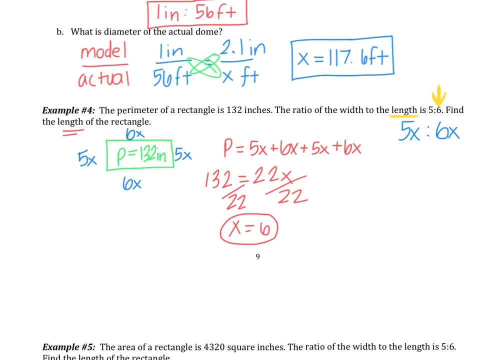 Because length came second in my ratio. that makes it the second value in the ratio, So let's plug it in. The length is really 6 times x. Well, I know that x is 6.. So the length is really 36,. 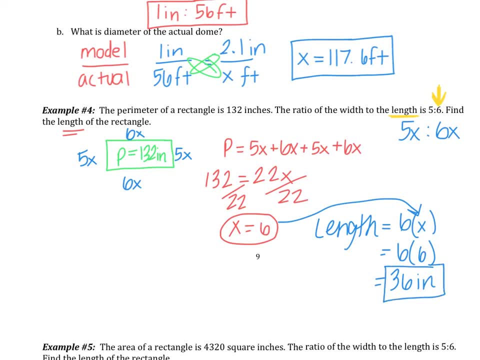 put your units of inches, Okay. you will see these again and again, so please be aware of this ratio. 5 to 6 does not mean it's a side length of 5 to a side length of 6.. There's some kind of ratio in there. 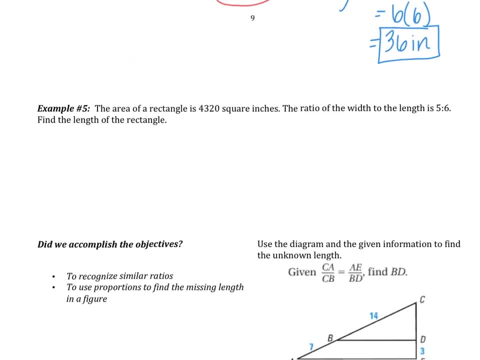 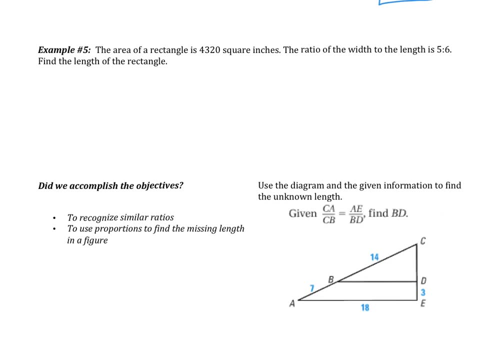 Okay, example 5: almost done This time. now we're talking about the area of a rectangle being 4320 square inches. The ratio of the width to the length is 5 to 6.. Find the length of the rectangle. Take a moment, try this one on your own.